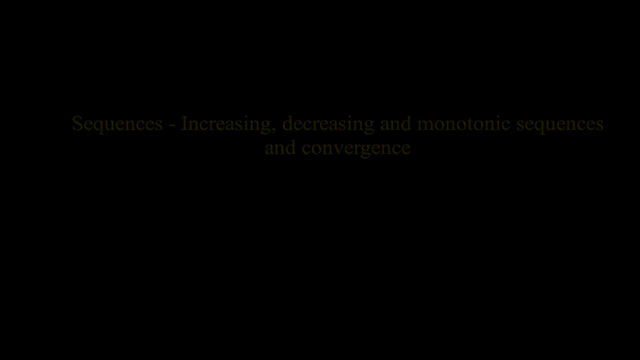 Okay. so next we want to look at the concept of increasing and decreasing sequences and the associated concept of monotonicity. So let's look at an example. So here we have a sequence: a, n, n equals 1 to n equals infinity. Okay, now if we have the situation that the 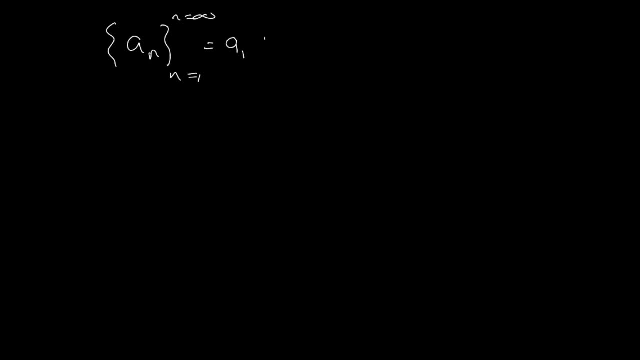 terms of the sequence, remember, are going to be a 1, and so on till infinity. Okay, they go on forever. So now, if we have the situation that a 1, a 2 is bigger than or equal to, greater than or equal to a 1,, which is in here, all the way to a n, which is again a n plus 1, 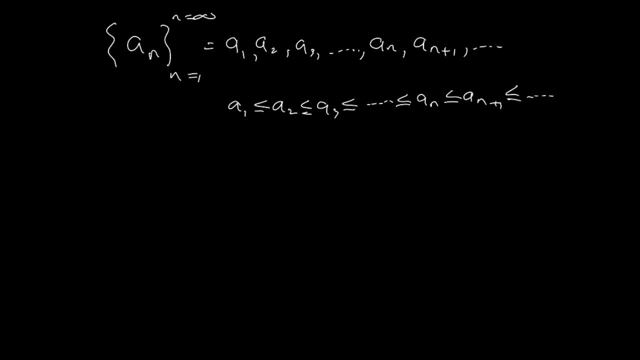 is bigger than that. And this goes: this relationship is going to be a n plus 1. So this relationship goes on forever. So that means that every term in the sequence, every new term, is bigger than or equal to the previous term. That means that the term seems to be. 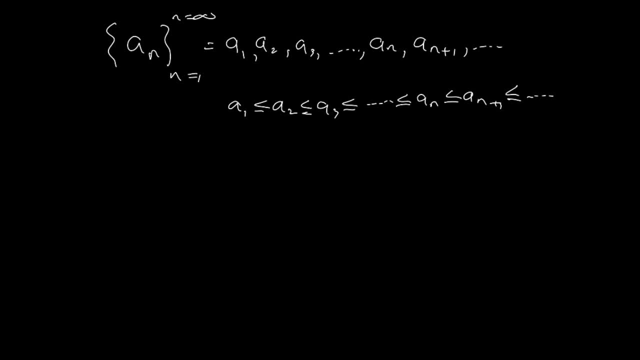 every term in the sequence is getting larger, which means the sequence is increasing. Okay, so sequence is increasing. if that situation occurs Now at the same time. if, on the other hand, these signs are all reversed and in fact we have this situation, 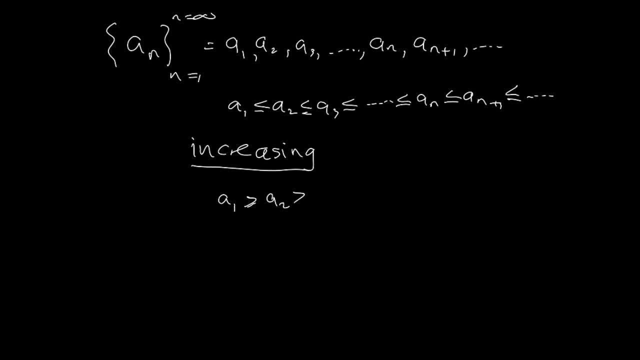 that a 1 is greater than or equal to a 2, which is greater than or equal to a 3,, which is greater than or equal to dot, dot, dot dot. greater than or equal to a n greater than or equal to a n plus 1.. In other words, the first term is the largest term, and then 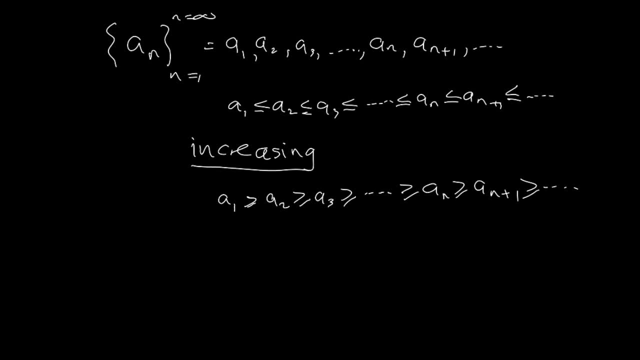 every term after that in the sequence is smaller than the previous one. So in that- and it has to be consistently that way for all, n? Okay, this has to be true for every single value. No value in the middle of the sequence could become suddenly larger or smaller. It cannot. 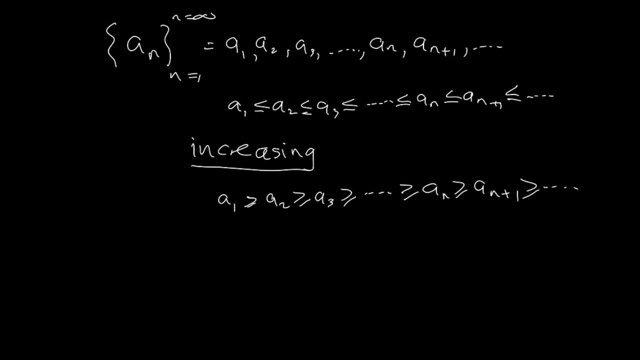 happen, All the terms have the maximum they can be is equal. Otherwise, in this second case that I'm looking at right now, in other words, in this case, all the terms, every single term, has to be less than this, has to be less than this. this has to be less. 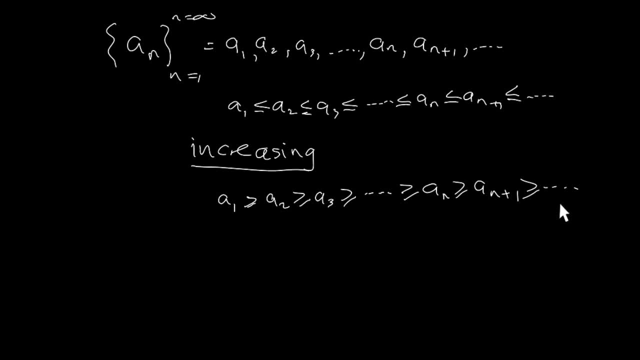 than this and so on, And none of these terms, none of the terms can become bigger than the previous term. It violates the rule. then Now, if that does happen, then we say that the sequence is of course decreasing, Because that's what's consistently happening Every. 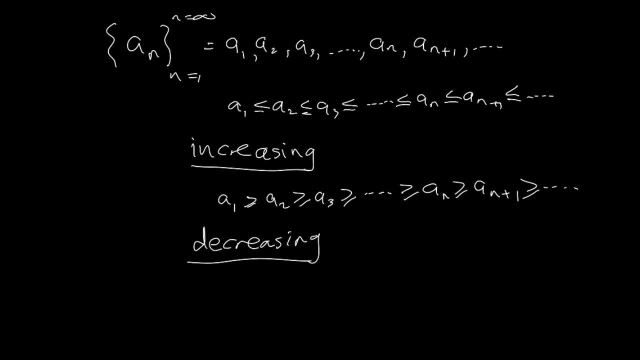 term. every next term in the sequence is less than the previous one, so we call it a decreasing sequence. Now, if a sequence is either increasing or decreasing, either one of the two, then it's heading in one direction. It's either increasing or it's decreasing. We call it. 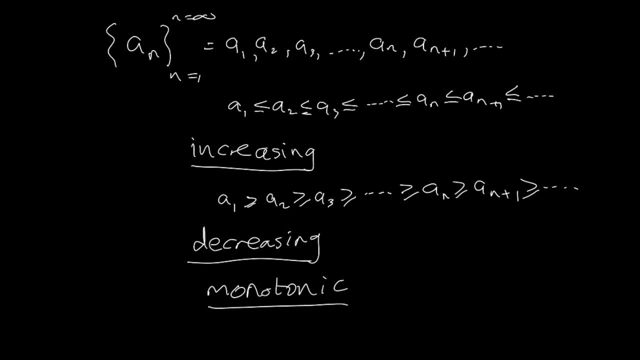 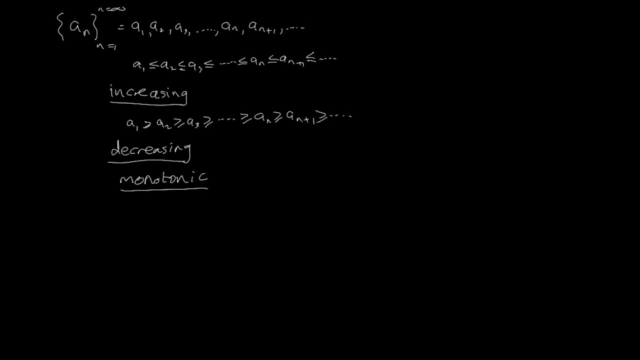 monotonic. okay, If it's increasing. either increasing or decreasing, we call it monotonic, okay. Okay, next concept, before we get to our result, is the concept of boundedness. So we say that a sequence, a, n, n, equals n, 0 to infinity, okay, is bounded. There is a number, some number. 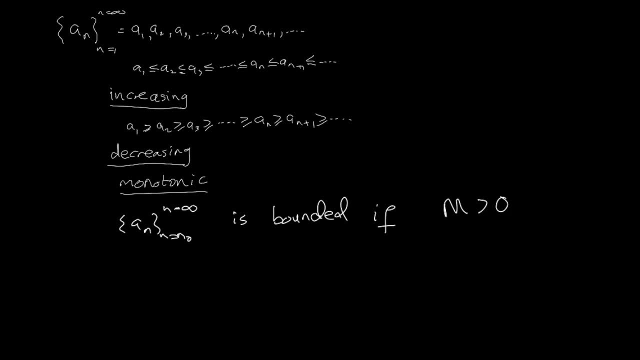 m, which is a positive number, okay, such that the size of a n, each a n, is less than or equal to m for all n, okay. So it means that this, there is this magic number, this magic number m, and it's a. 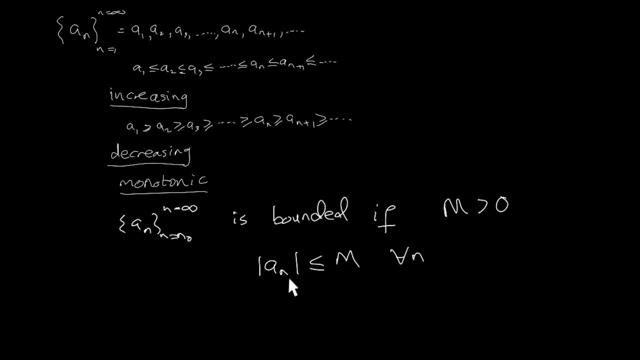 positive number and all the terms in the sequence. the absolute value or the size of each number in the sequence is less than or equal to m. It can never exceed m, So m is it always. the numbers will stay within, within this bound. within this bound, Then m is called the bound. okay, We call m. 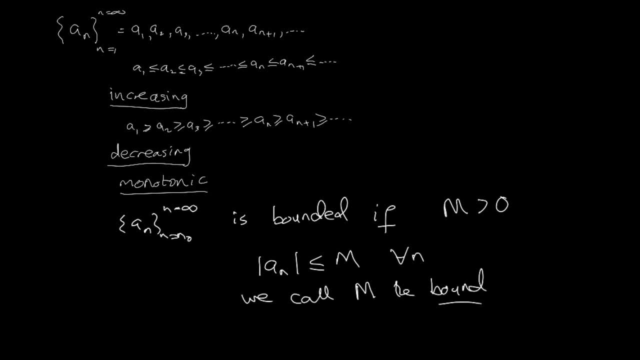 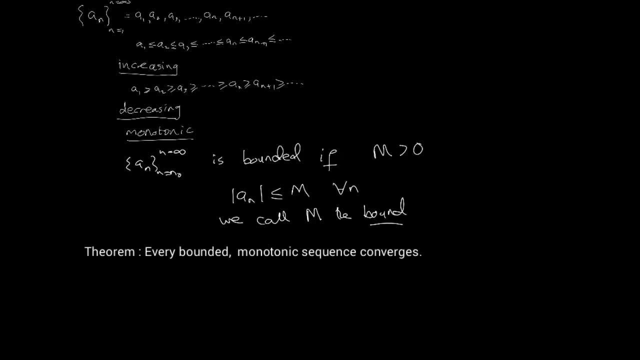 a bound, or the bound as you wish. okay, So we say: a sequence is bounded if there is such an n. Okay, so we have our theorem now: Every bounded, monotonic sequence converges. So if a sequence has two properties- one it is bounded, two it is monotonic, then the sequence converges And it 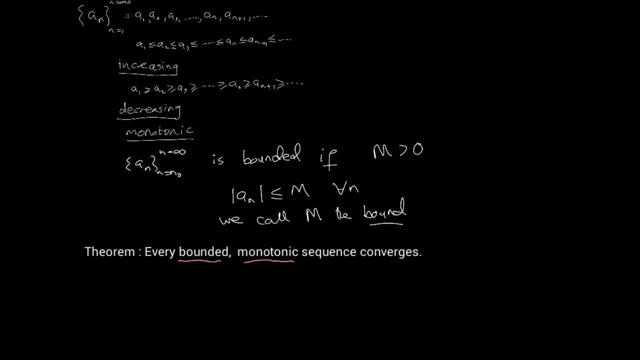 makes sense if you think about it. Obviously, if a sequence is increasing or decreasing, it means it is monotonic. Now if it keeps increasing, for the sake of argument, let's, let's see a graph here, for sake of argument. So suppose that a sequence is increasing, So increasing, increasing, increasing. but there is. 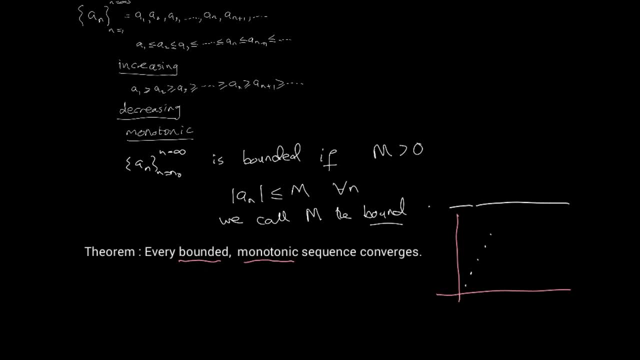 a bound, m, at some point, So the values will never get above that. So, and then they start slowing down because they can't go above the bound And they're monotonic, so they can't decrease anymore either, So they will stay. 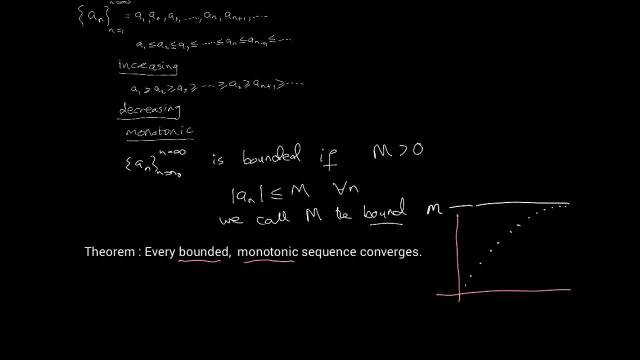 Slowly increasing or remaining the same till they actually reach this bound, m. And what does what does that graph tell you? It tells you that the sequence is converging to m, in fact, okay. Or if it doesn't converge to m, it's going to converge to some number pretty close to m, okay. 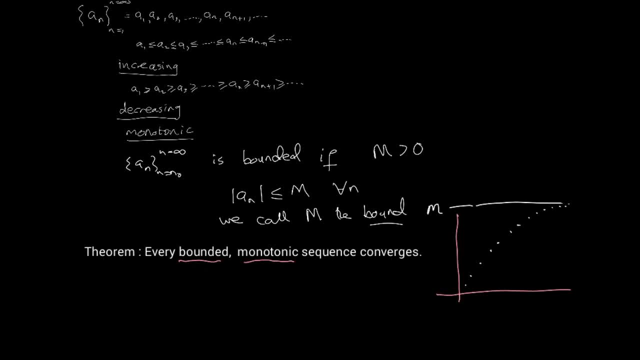 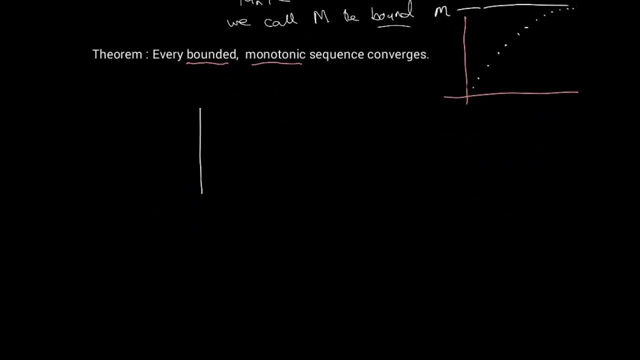 What's happening is now. let's let's look at the case of a decreasing sequence for the sake of argument. So let me do another graph for you here. So that's the case of an increasing sequence. Let's look at another graph. In this case. let's look at…. 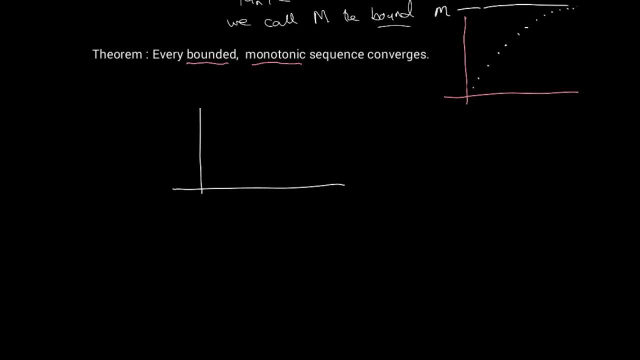 Suppose there is a bound m here. Now, one thing you must keep in mind is that the bound we're talking about, we is a positive number, number one, okay. And second, the sequence can have negative terms, But the absolute value of this negative. 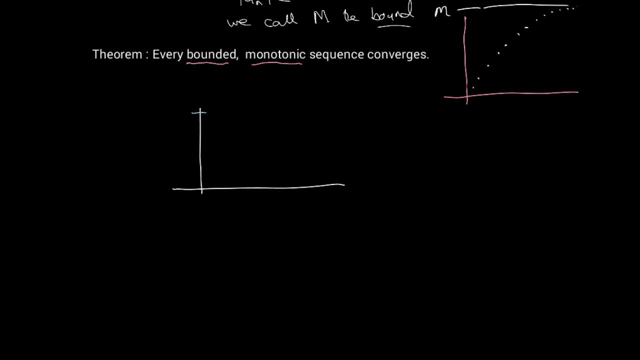 this negative term will be bounded, okay, will be bounded. so, for instance, now, if it's monotonic though it could be, for instance, it could be negative, no problem. okay, then what will happen is there will still be a bound at some point. okay, if it is bounded. if it is bounded and 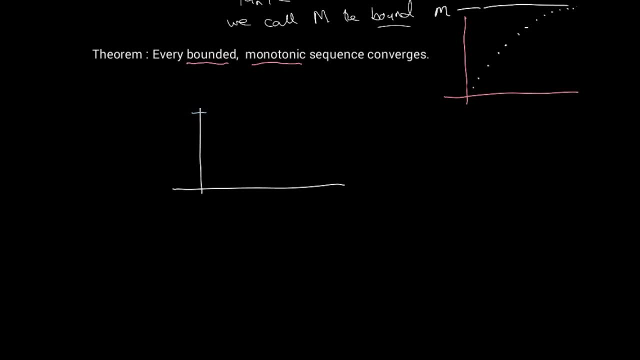 it is monotonic, then it will decrease. obviously it will decrease. now, if it's decreasing, for a second i'm going to show you two graphs. okay, so here, suppose that it starts at a certain point and then it starts to decrease and decrease and possibly it even crosses the axis and becomes.